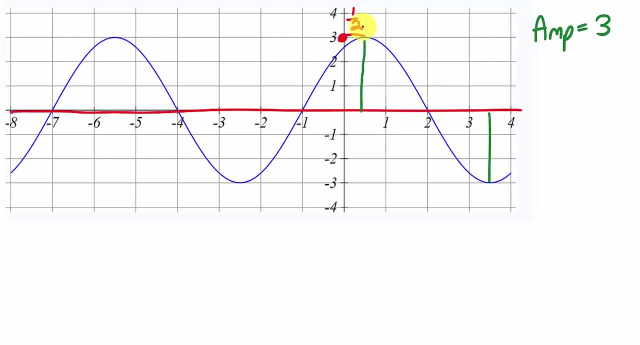 what I'm going to do. I'm going to use a cosine function, So I'm going to have y equal and I'm going to put three, because that was the amplitude, and then it's going to be cosine. Now, right here, I need to figure out the period, and I know there's nothing added on the end because there was not a vertical shift. So what is the period? and if I look, I can look at. maybe I'll just look from maximum to maximum here and I'm going to 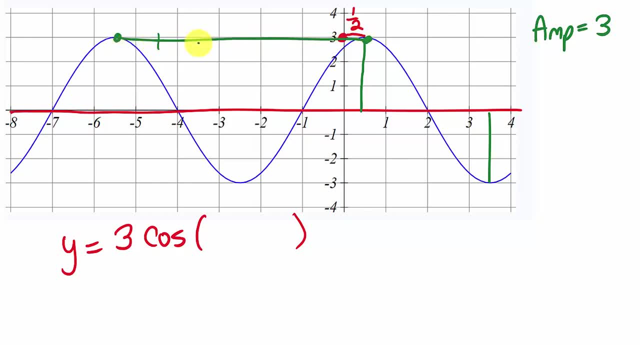 see how far apart those are. So it looks like that's going to be one, two, three, four, five, six units apart. There's no pi on those, and so the period equals six. So if I had two pi over omega, I'm going to get six. So we know that omega is going to have a pi in it and it's also got to have a number, so that when I combine those I get six. So that's going to be pi thirds. 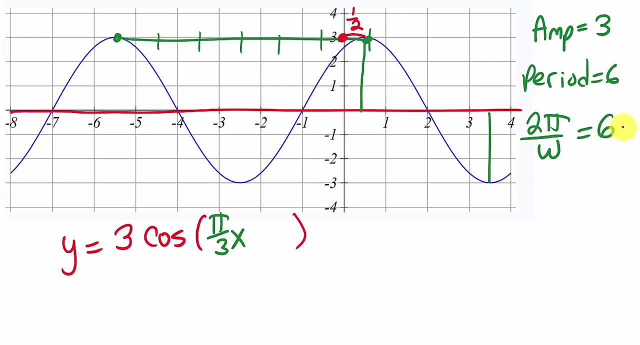 x. And again, if you don't see that in your head, it's easy to solve: Multiply the omega here and then divide the six. So two pi divided by six equals omega and that reduces to pi thirds. Now we said that the shift was one half. I'm going to call that PS for phase shift. The phase shift was one half. Now if I just put minus a half here, that's not going to work unless I put it in parentheses, and I have it. 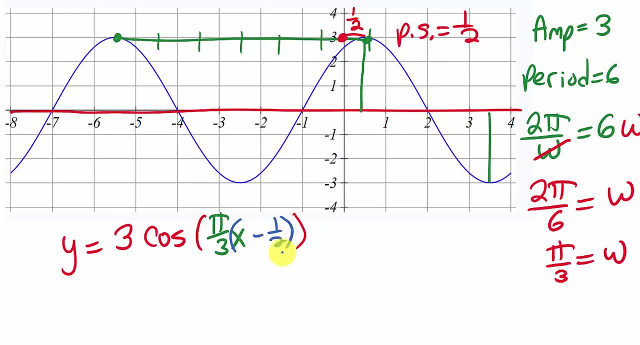 minus one half, like this. So that's one way I could leave it. so the phase shift was one half. If I needed to express it without any parentheses, I could distribute that through and it's going to be pi thirds x minus pi sixths. And we could just run a quick check on that, because if I set this equal to zero and solve it, I should get that phase shift of one half. and you can see, indeed I do, because I have pi thirds x minus pi sixths. 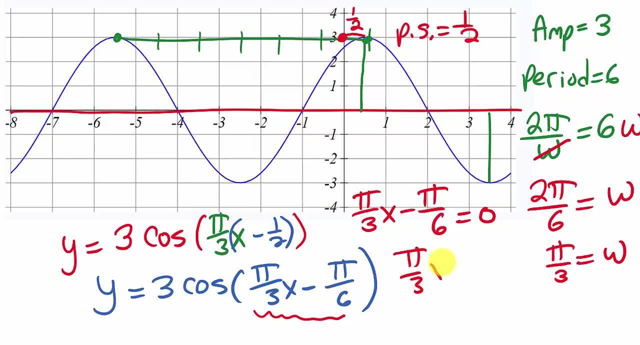 So pi thirds x equals pi sixths, and dividing by pi thirds is like multiplying by the reciprocal. So let's do that over here. You can see the pi's cancel and I'm left with three sixths, which is one half. So here is the equation of the graph shown.